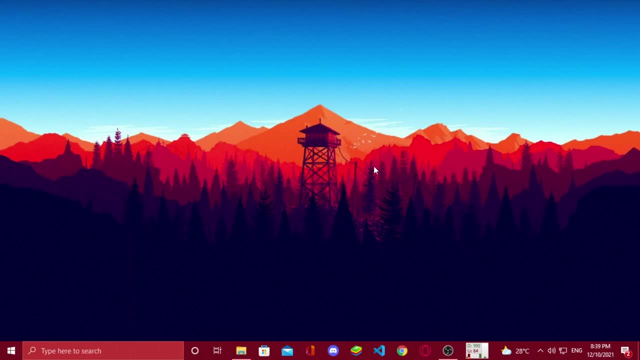 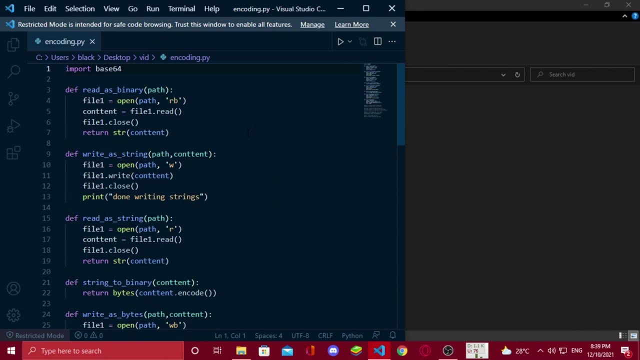 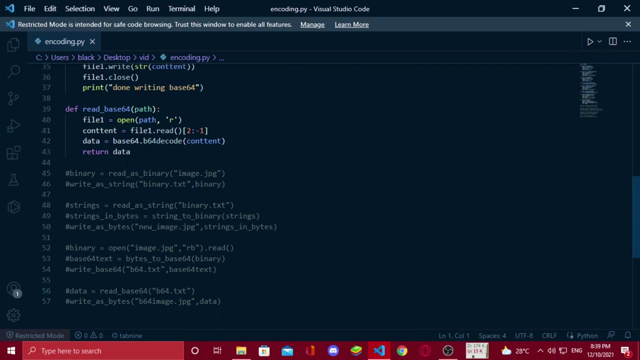 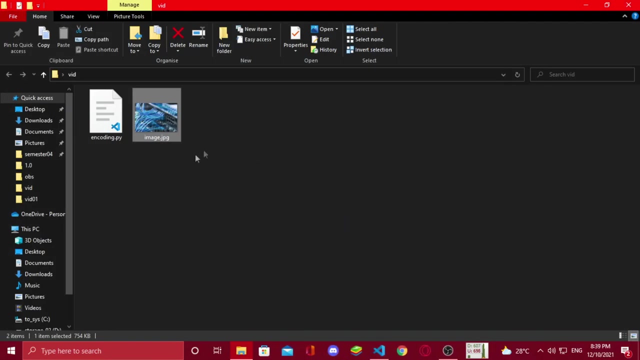 Otherwise the program gives errors. First let's see about this encoding. Here I have made Python script. I'll open it. You don't actually have to understand this Python script, I'll just say what it does. You only have to understand what it does. And there is an image here which is this one: 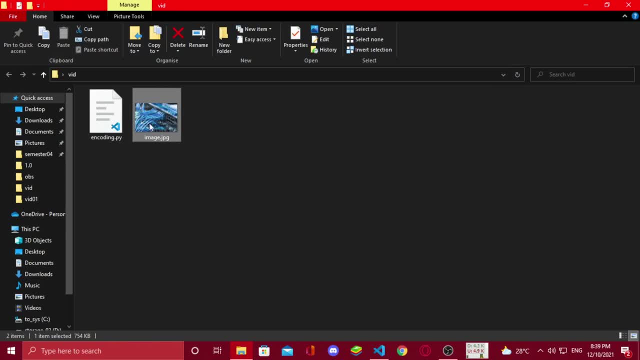 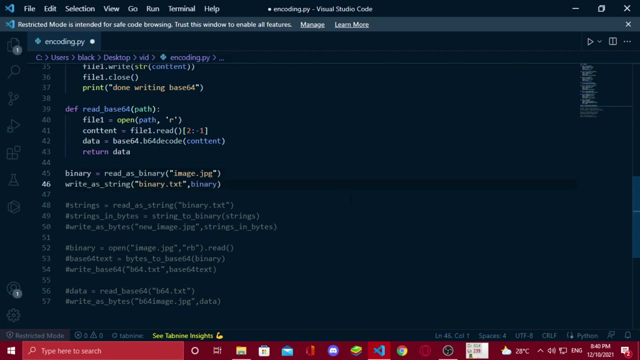 And now I'm going to convert this image into string. Actually, what I'm doing is I'm reading this image in this Python script, I'm writing this Python file as a bytes object and then writing those bytes into a text file. Let's see how to do it. I'm uncommenting these two lines. 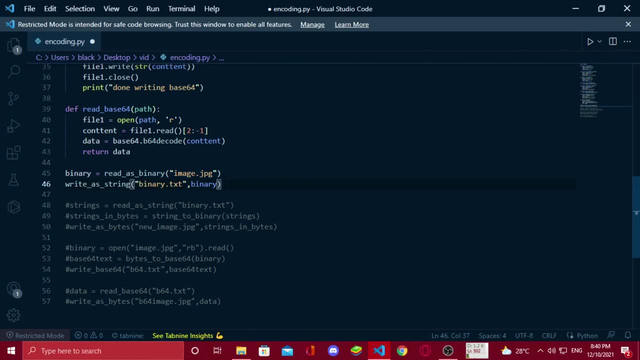 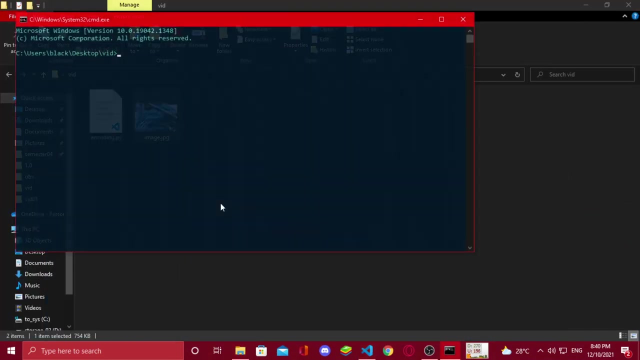 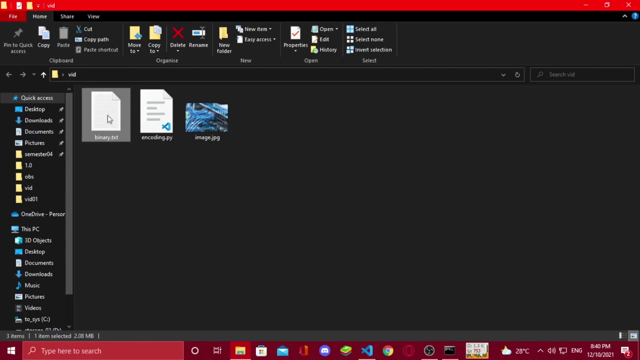 First it will read the image as a bytes object. Then the program will write those bytes array into a text file named binarytxt. I'll save it, Then I'll run it here. It says: done writing strings. And there is a binarytxt named txt file. 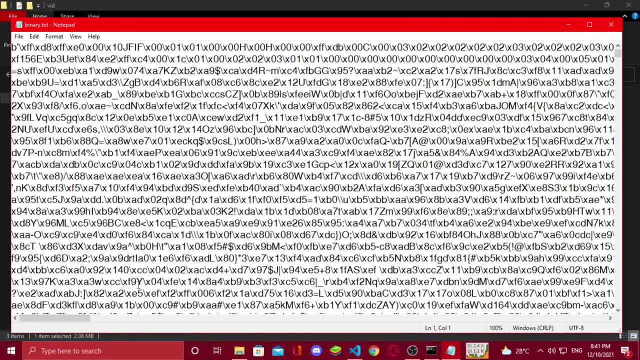 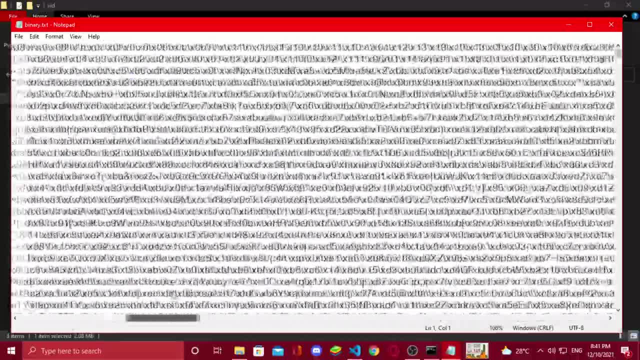 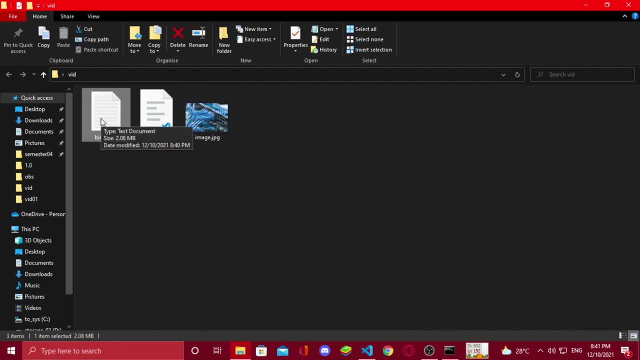 Let's open this And you can see there are so many characters here. This, actually we cannot understand what is going on here. But Now let's try to write these bytes into a jpg file named new imagejpg. What does that mean is? 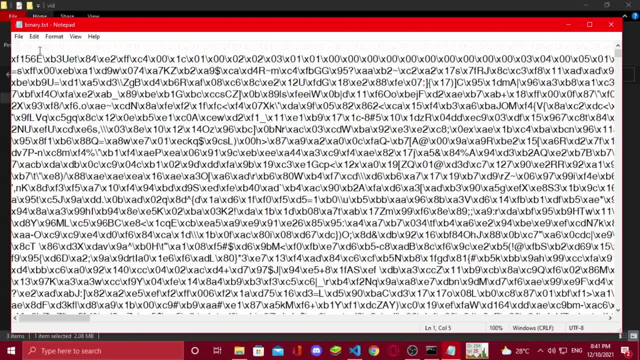 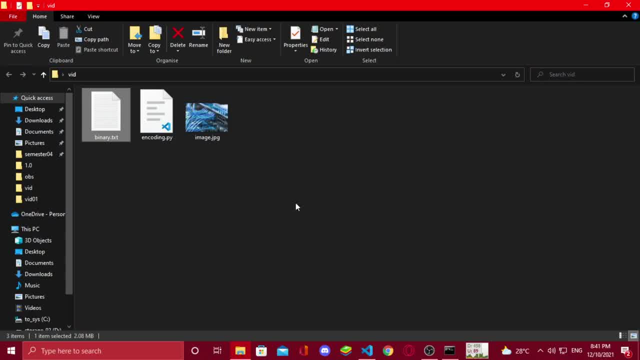 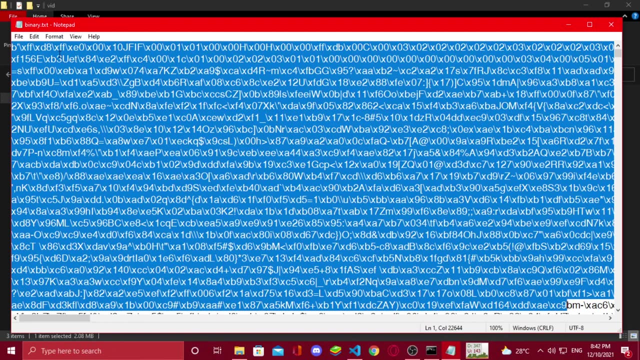 First it reads all these text from this text file And then it converts these strings into bytes, Then it writes those things back into a jpg file, Those things back into an image file, Which means I'm basically trying to get this image back using these strings here. 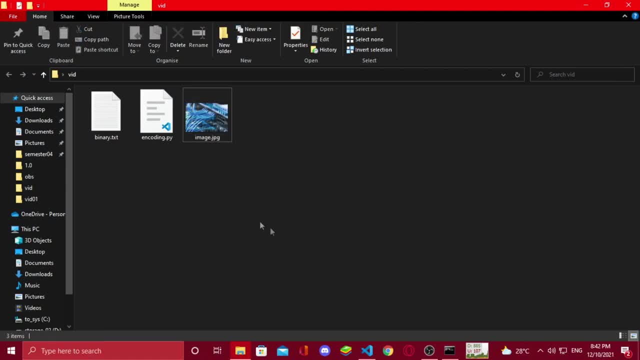 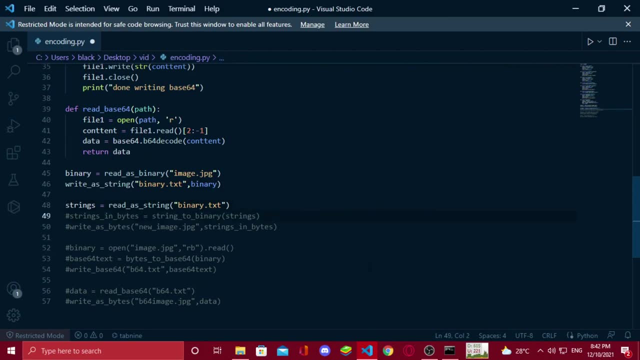 Using this text. I'm going to generate this image again. Let's try this- And I will commit these two lines back Now. basically, what it does is it reads that binarytxt text file, Then it gets the string into this strings variable. 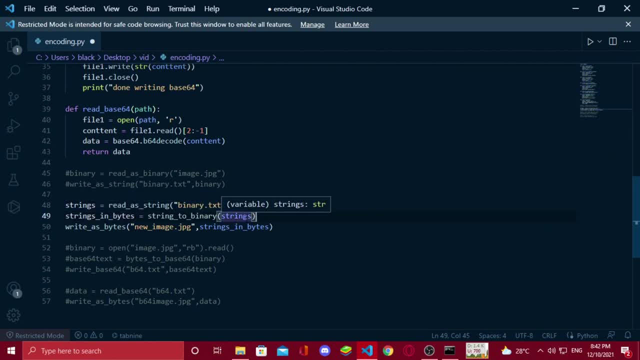 Then it converts those strings into data array- Sorry, the bytes array, Which means Then this strings in bytes variable is a bytes object. Then it will write those bytes into a file called newimagejpg, And let's see what will happen. 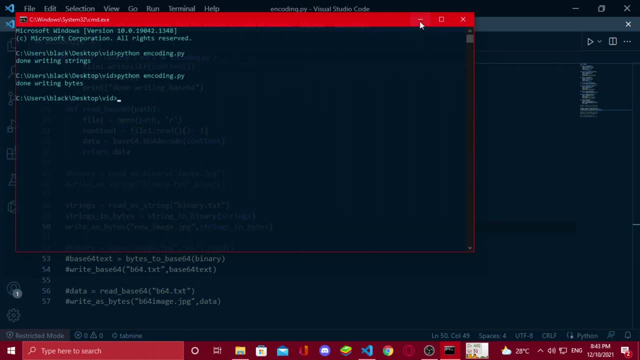 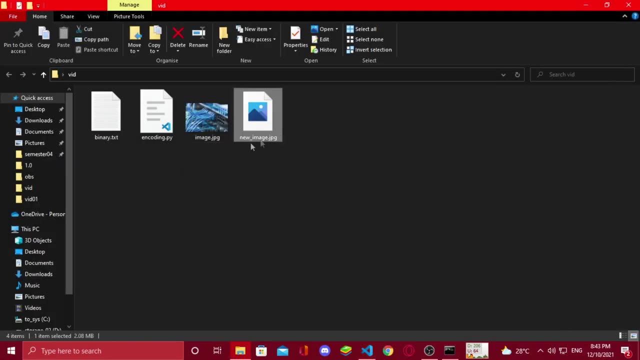 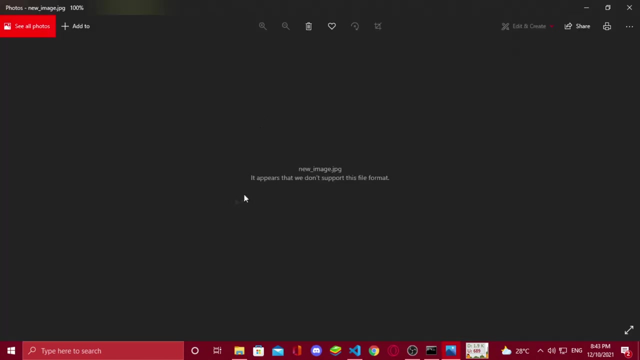 Okay, it says done writing bytes And there should be a new file called newimagejpg. Let's see, There is an image But, as we can see, it does not show the thumbnail And if we open this, it gives this error. 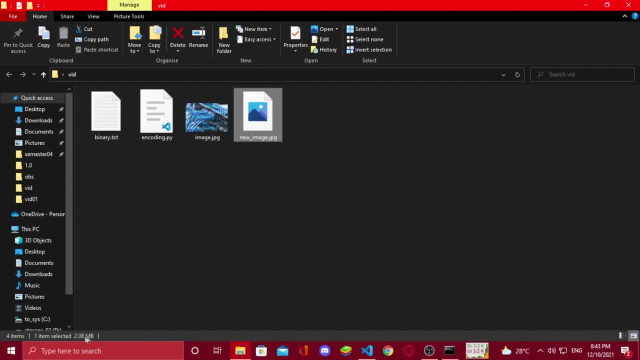 And also if we check the sizes of this image, This is 2.08 megabytes And this is 754 kilobytes. So these files are different, Which means if we read some file in bytes And if we write those bytes into this kind of text file, 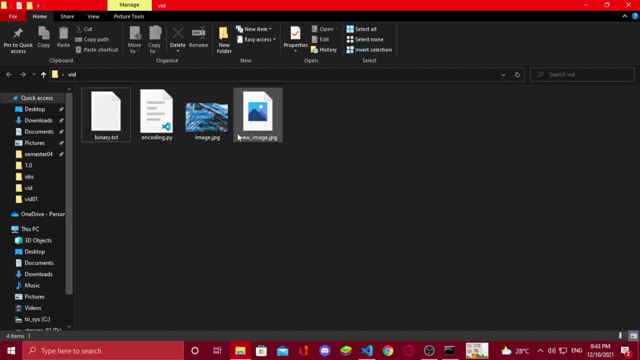 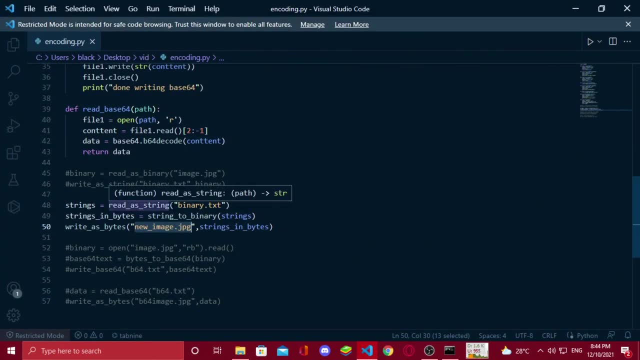 We cannot get the same file back By writing those bytes into that object in this python directly, But there is a way we can do this. We can use some kind of encoding into this string. I am using base64 encoding here, And now let's see how to do it. 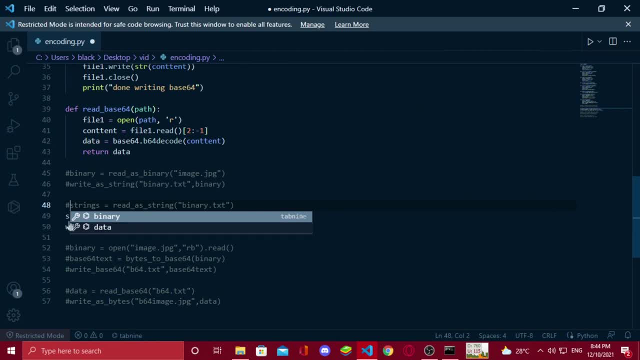 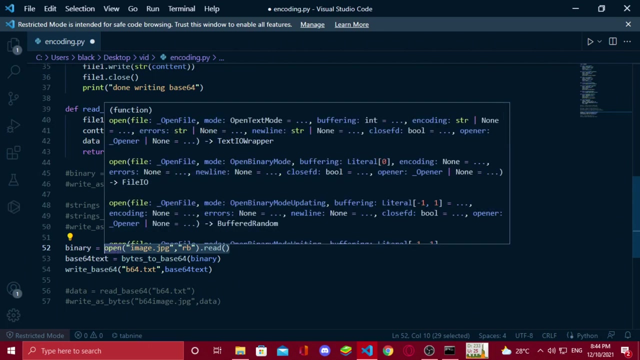 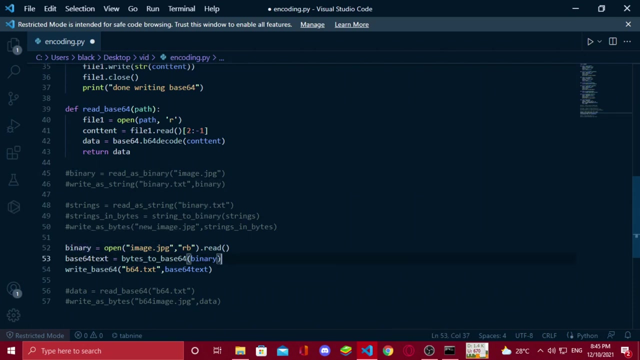 I will comment these lines again Now. I will uncomment these three lines. Now, what does this do? is It is opening this original image And read this as bytes. Then it takes all bytes into this variable. Then it converts those Contents into base64. 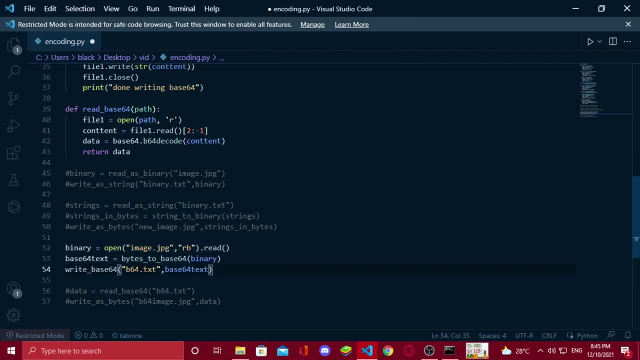 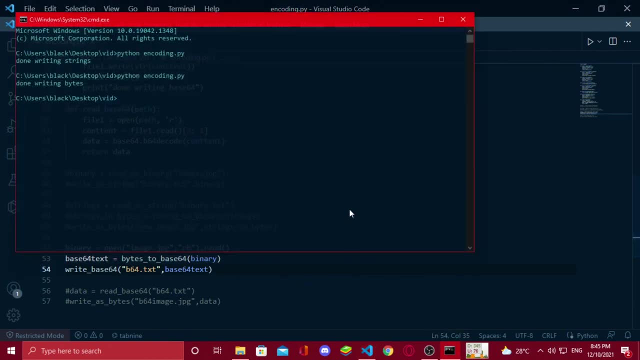 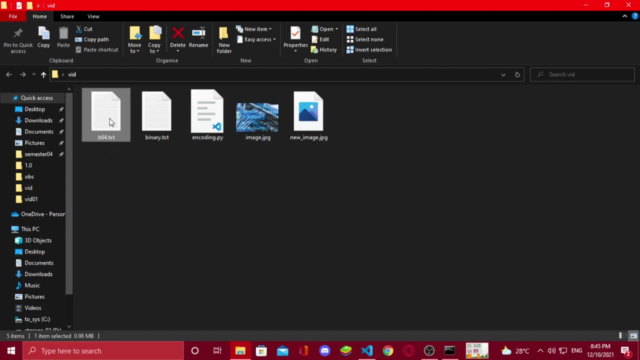 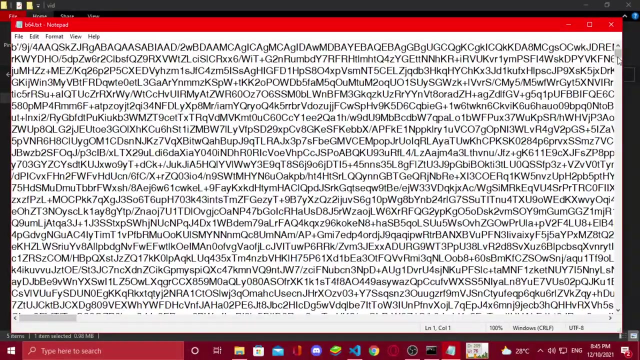 And it writes those base64 string into b64.txt text file. Let's run this. It says done writing base64. And there is this b64 text file. If we open this, There is another weird string, Weird text. We cannot understand what is going on here. 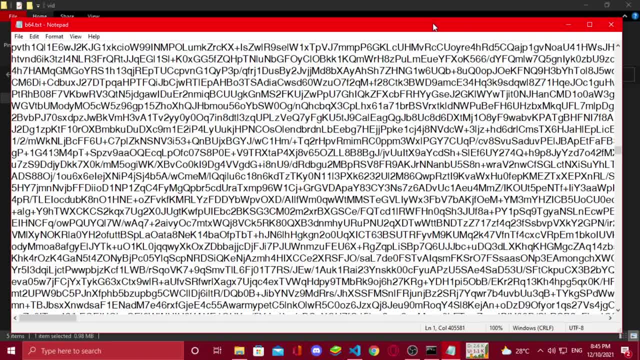 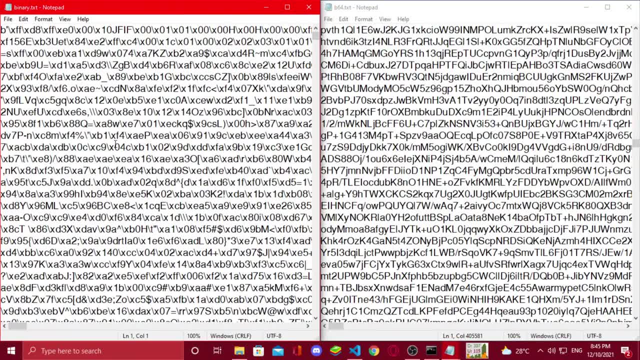 But this is different from the last one, This binarytxt. As you can see, there are so many slashes And x characters, Zeros and numbers. There are so many things, But in here you can see there are numbers and English letters. 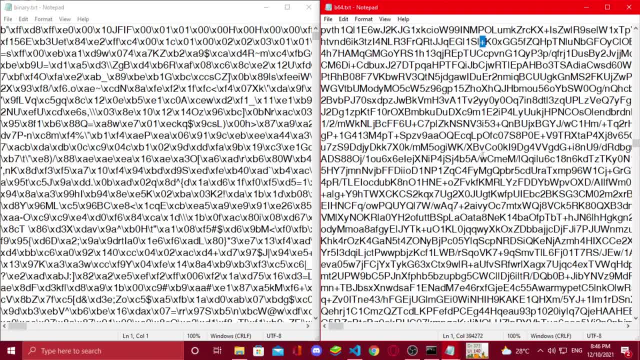 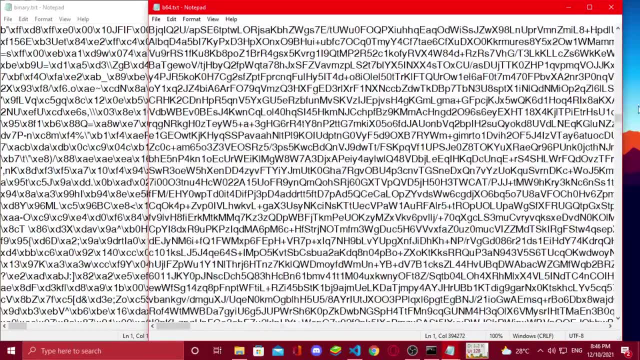 Yes, there are some Plus, Minus, Inverse, Two, But there are no those. There are no those Double quotation marks And quotation marks. Of course. there is one quotation marks Mark on the beginning of the text And the end of the text. 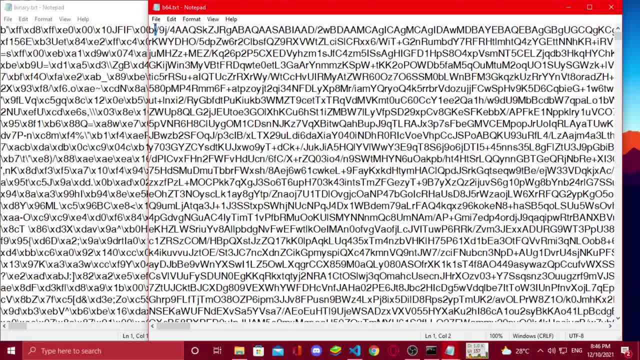 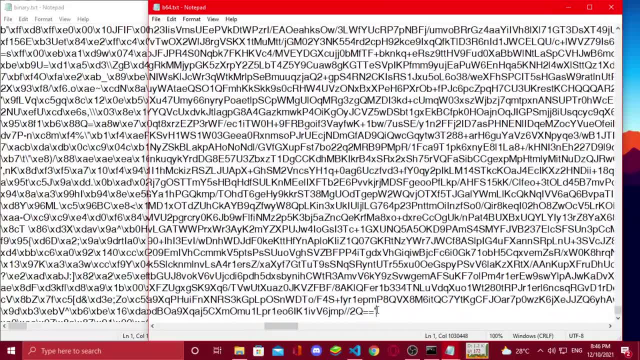 Other than that, there are no any quotation marks. This one, And at the last of the text there is one, Two. This is it. Other than those two, There are no any quotation marks, So we can use this text inside our program. 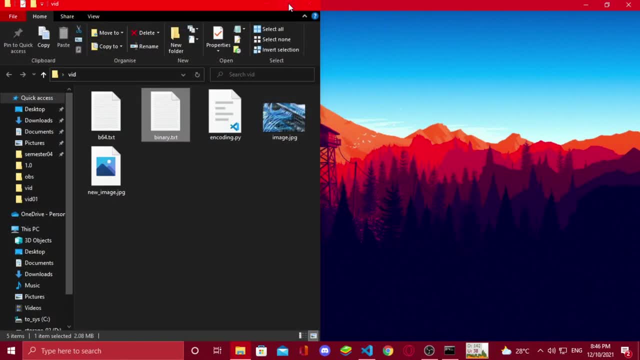 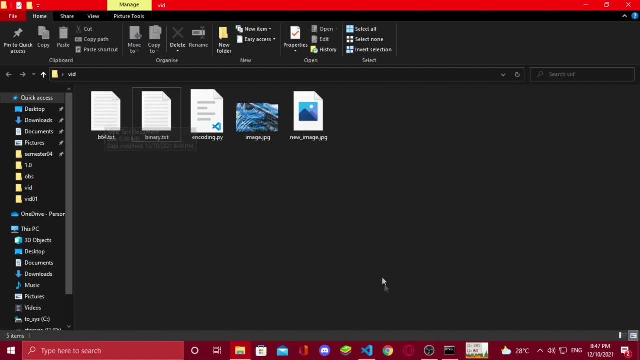 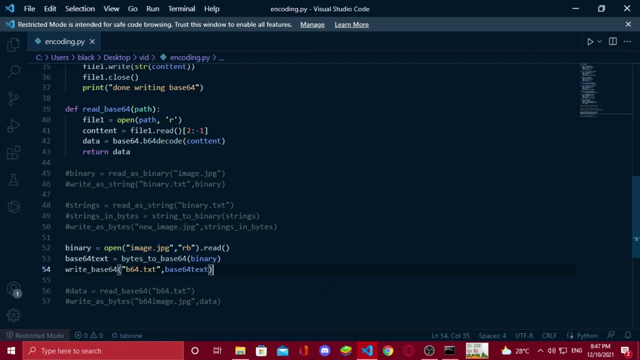 Okay, That's the base 64 text. Now let's try to write this base 64 into a new file. Actually, there is no mean. It does not work. If we write that base 64 text directly to a file, We have to convert that back into binary object. 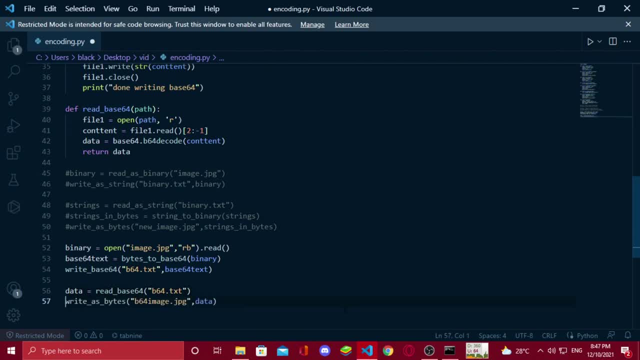 Here is those two lines. I will uncomment those And I will comment these three lines back. What does this do is, First, it read that base 64 text And convert that into binary object. If we go to this readb base 64 function. 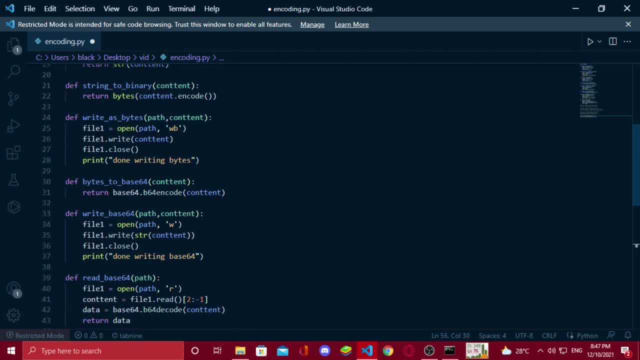 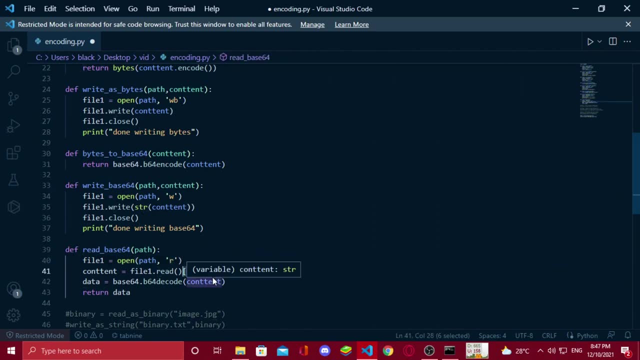 Where is it? It is What it does is It reads the file as a string, Then it takes the content from Second. No, The first. Now the second means From the third character to last character. But last character is not included. 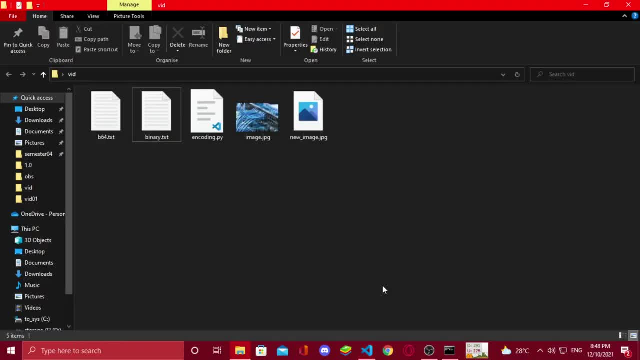 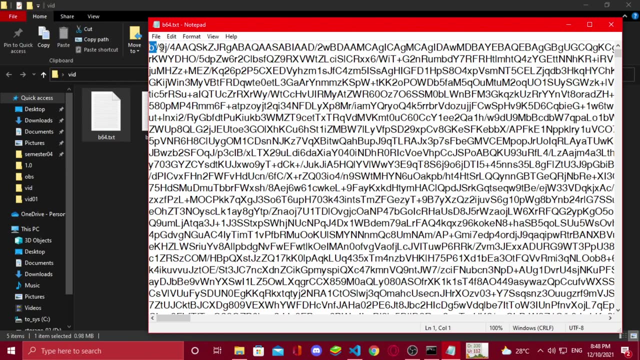 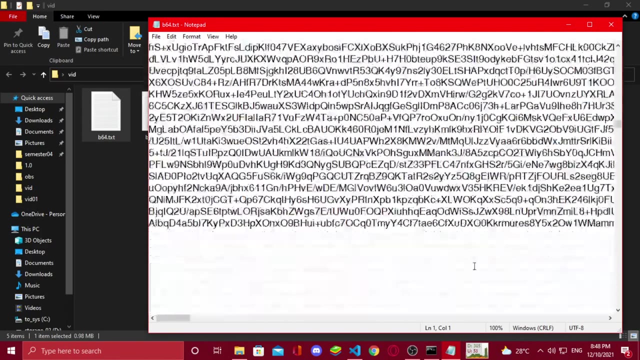 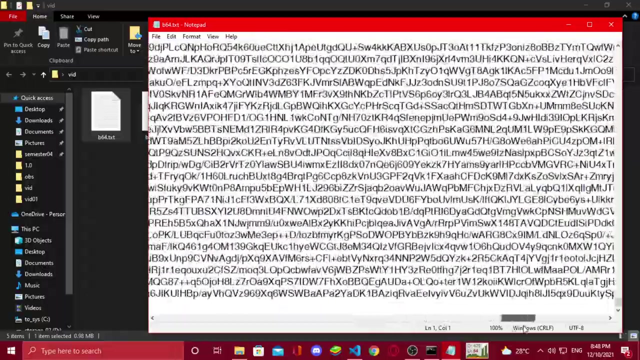 Why we do that? That's because There are those Simple b And this quotation mark. We have to remove this. This is Default python output. There is a, b And That Last quotation mark Which I showed you earlier. 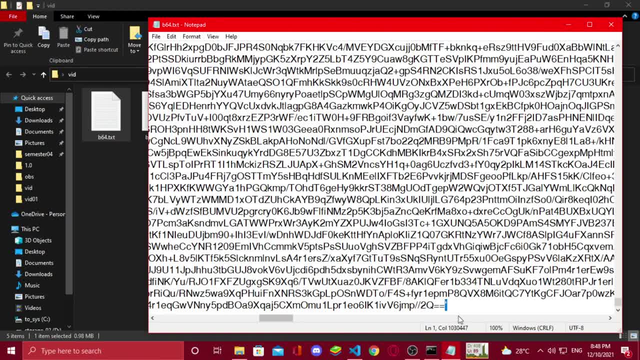 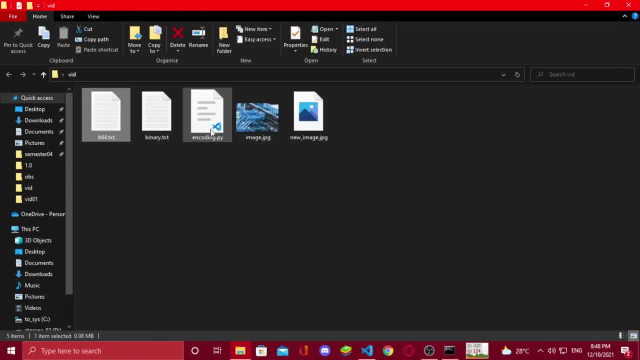 This one. This is because When we encode something in python, It does this And we don't want Those Simple b And quotation marks, So we To remove those. We use this. It only gets this range And. 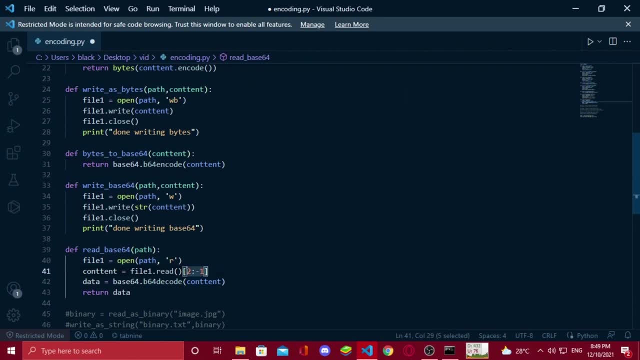 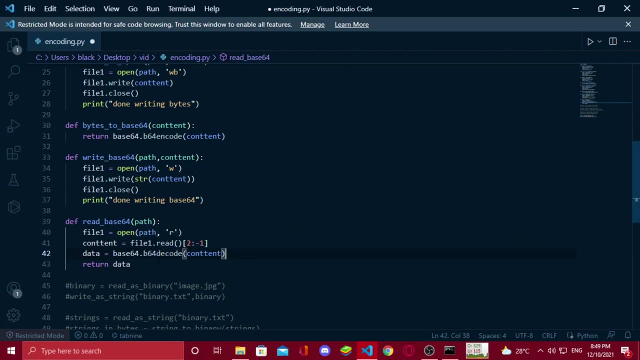 And this line will Decode the Base Base 64. String Into its original Format And it will return this Data Variable. And that's it. So That's it. Thank you For watching, See you. 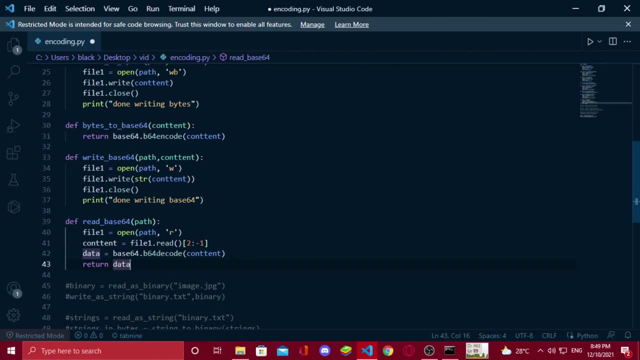 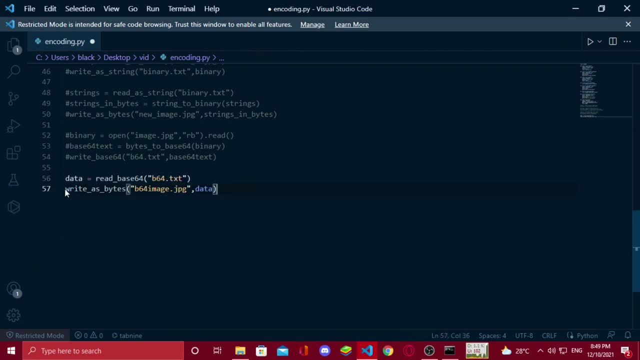 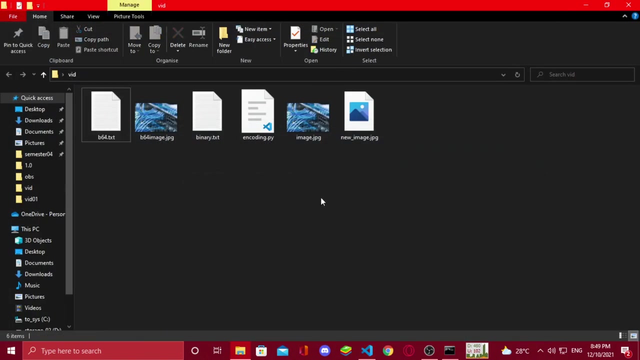 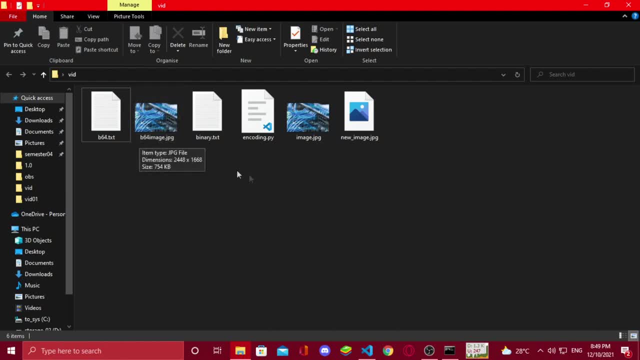 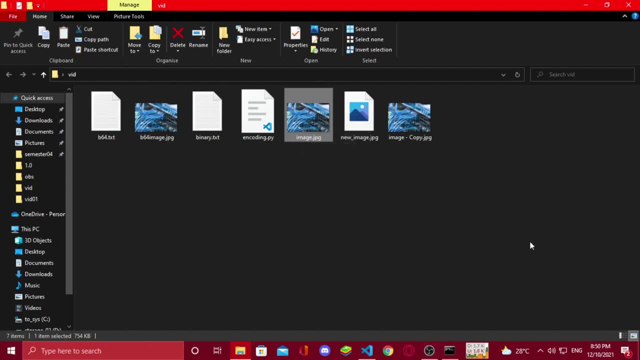 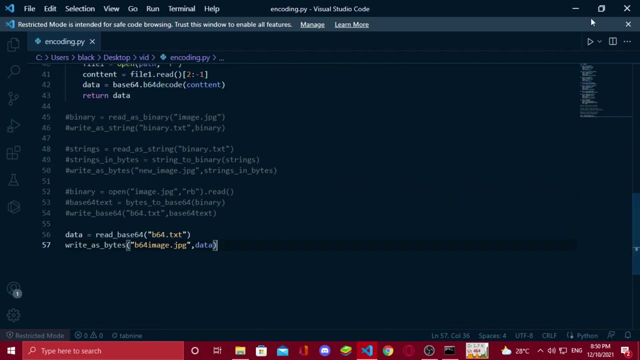 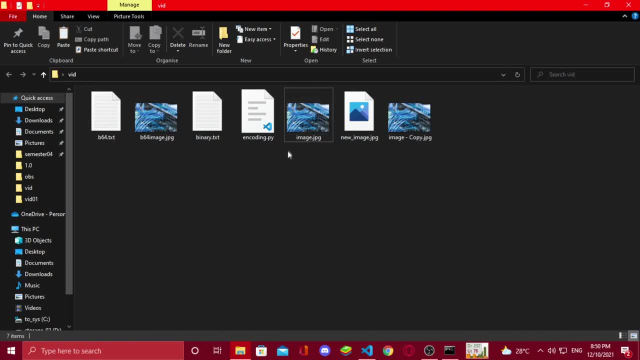 most basic way of doing it, and that is a. that is the first use of cryptography that i'm explaining today. i already explained that, and now let's talk about another thing. uh, now let's talk about encryption. the first one is: i'm going to. the first one, i'm going to. 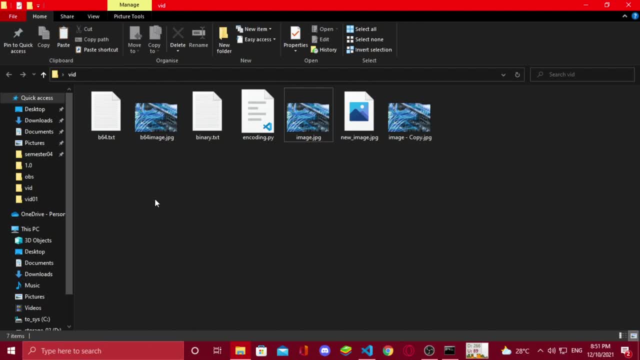 describe this? uh, actually i'm going to describe this. the first example i'm going to show you is the whatsapp encryption method. actually, it's not a whatsapp encryption method, whatsapp message encryption type. first i will connect my phone to my computer and then you. i can show you the internet file system and show how those files are stored in ufo. this is my mobile. 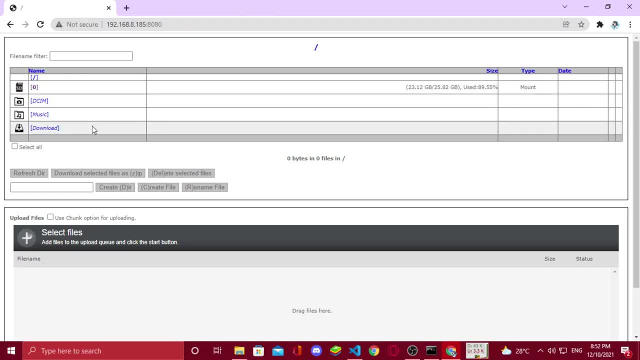 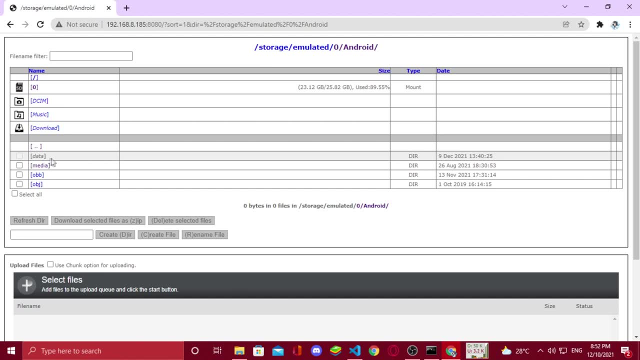 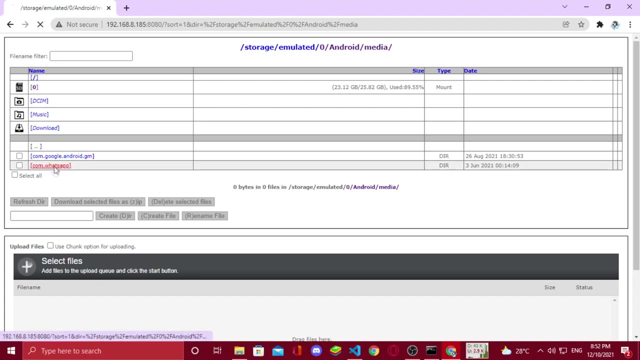 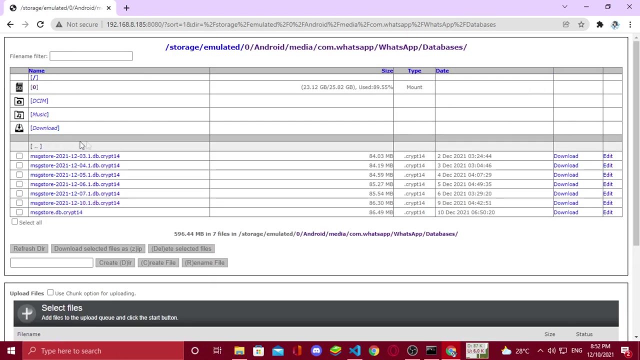 phone's file system, it is the internal storage, and if we go to this zero, then there is android it and there is media, and here you can find this comwhatsapp folder. there is whatsapp again, and in these databases, these are the whatsapp messages that are backed up on your whiteboard, as you know. 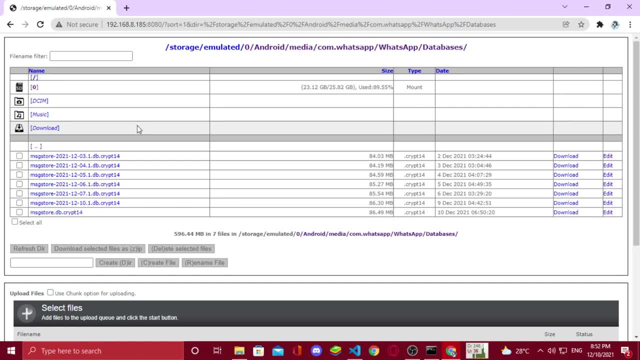 that when we are installing the whatsapp in a new device, it is asking us for if there are any backups. if there are any backups, what it does is it is reading these files from your sd card or something, and i will download one of these files into my docker computer and let's go to downloads. 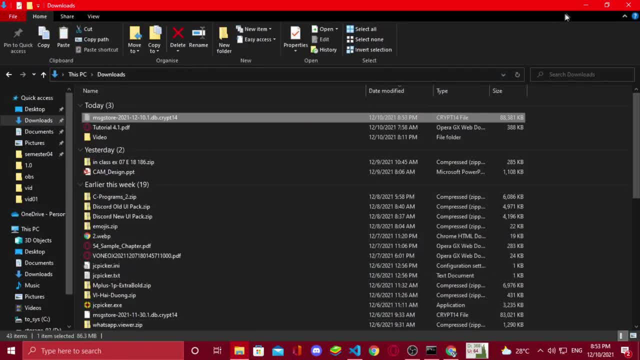 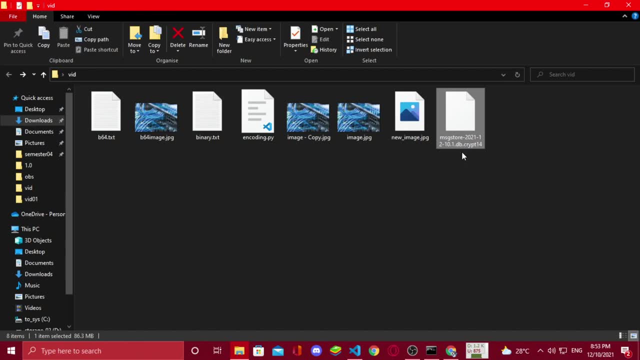 and i will move that into my folder here and, as you can see, this file is in a different format, which is encrypted, and it is not a text or any kind of document or pdf or something like. it is in crypt 14 format, which is basically encrypted messages. if i try to open it with 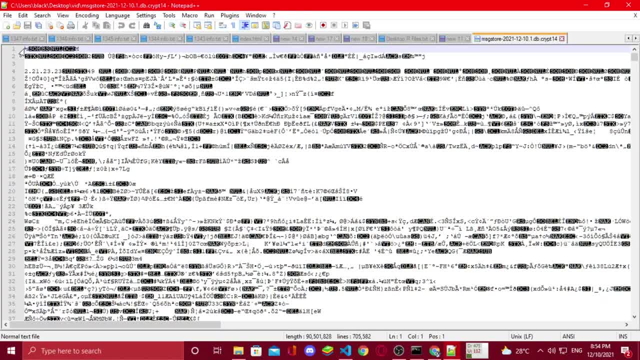 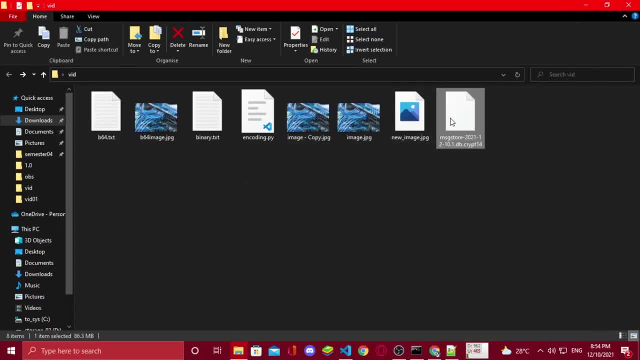 a notepad, it gives me this kind of nonsense test, and that is because this is encrypted and without knowing the key of this, the cipher, which is the encrypted method, we cannot reverse this. usually the key of this file is stored on your mobile phones data folder, which is the called the apps installed in that. 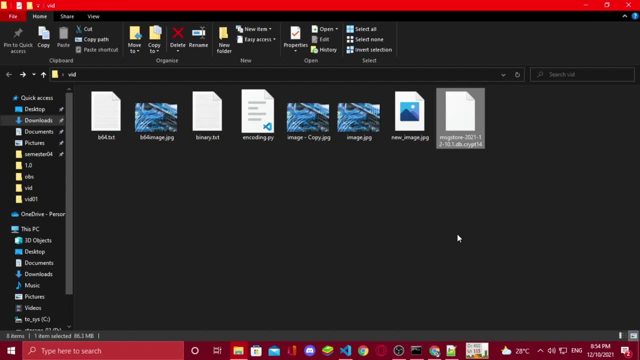 folder. there is data, then data, then there will be comwhatsapp folder, then there will be a. there will be a another folder called files and in that files folder there will be a file name key and that is your key. then that key is differ from user-to-user, and that's about that, whatsapp. 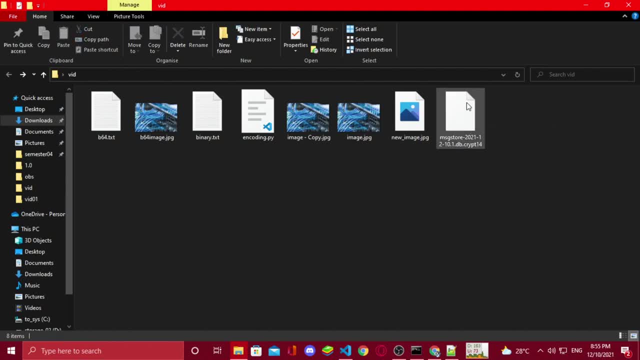 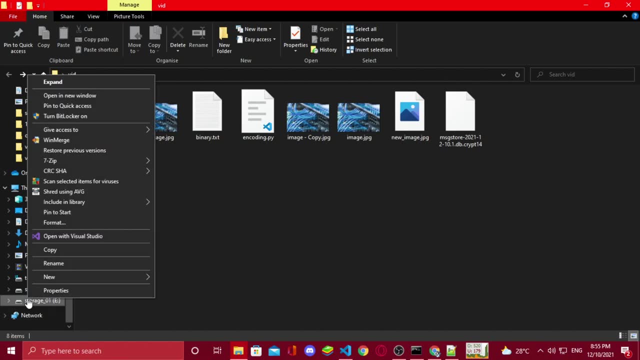 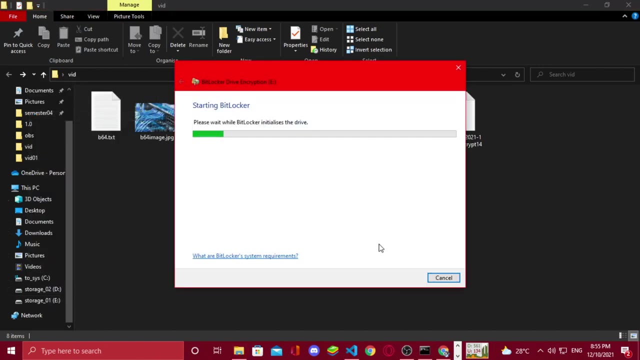 encryption. now lets talk about another type of encryption. if you go to here and if you right-click one of this drives, there is this turn between logo and it is starting, and this is also encryption. a very good example for people. what does this do? is this thing? 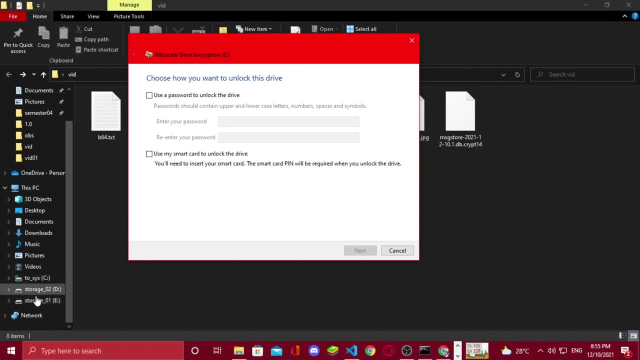 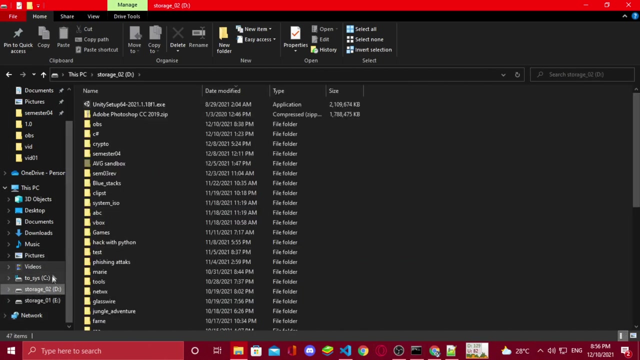 will encrypt your storage devices- sorry, the drives here. if I want to encrypt this D drive, I can click use a password to unlock device to unlock this drive and continue. but I'm not going to do that. but if we did that, what will happen is this drive will be encrypted and each time when we want to go into